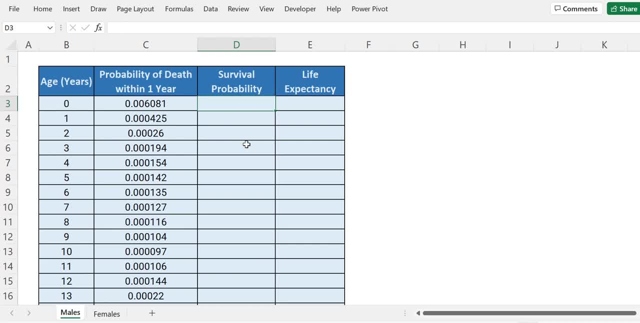 Hi everyone, in this video we will see that how we can calculate survival probability and life expectancy in excel for both males as well as females. So we are given with this data, that is, age in years and the probability of death within one year. So let's say, if the age of an 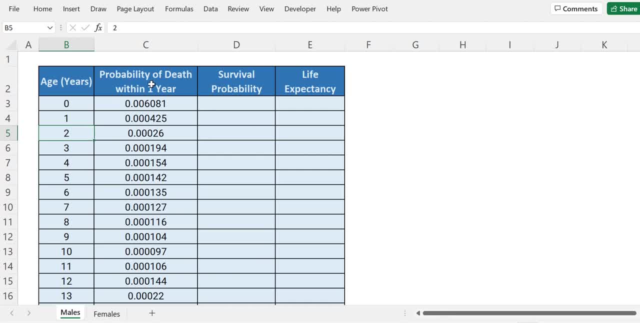 individual is 2 in years, so his probability of death within one year will be 0.000194. right, And now we have to calculate survival probability. So for calculating survival probability we have to assume one thing: that if the age is 0, the survival probability is 1. right, 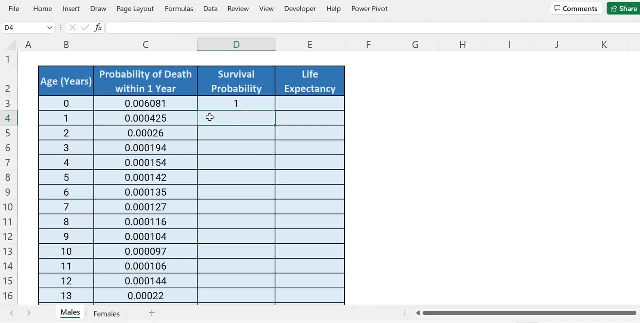 And now let's say for age 1, the survival probability will be the probability that he survived until age 0, that is, 1 here, and the probability that he will not die within next one year. So the probability of not dying within next one year will be: 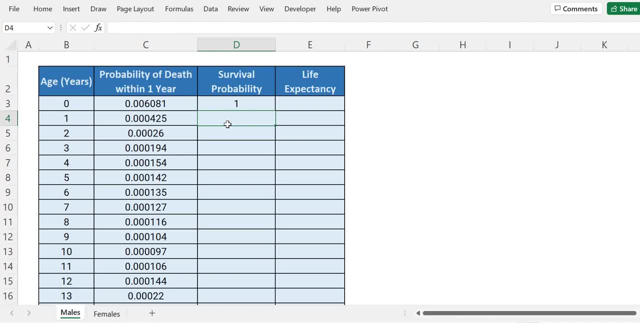 1 minus probability of dying within next one year. right, So they are mutually exclusive. So what we will do is equals to 1 minus this probability. So this will be the probability of that person not dying within next one year, correct, and with this we will multiply. So we will close. 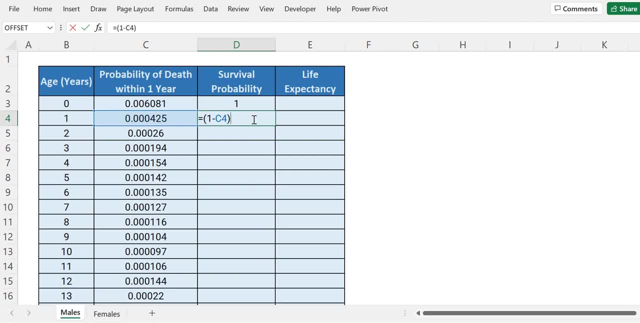 enclose these, this calculation in brackets, and with this we will multiply this particular survival probability, that is, previous survival probability. Press enter and we have survival probability for age 1, let's drag this down And we have corresponding probabilities of survival until age four. let say So, this is the number and this is for age five. Now, this we have to drag. 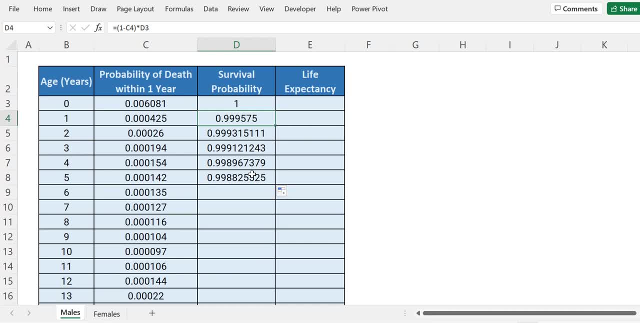 down, but we will now wrap this whole thing inside an array formula and we will use scan function for that purpose. So let's remove this, and now we will use scan function. so equals to scan and an initial value will be one. if you remember, if his age is zero, so the survivor probability will be one here. so that's. 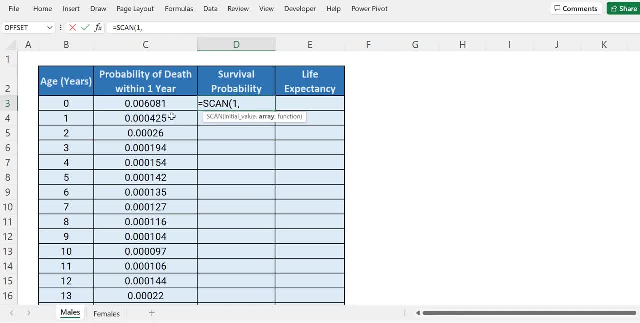 why initial value will be one and our array will be this array, this array of age right, and our function will be lambda. and let's say, our previous value is x and our current value is y, and now we will start writing our calculation. so what we have to do is if y equals to zero, so that is, if. 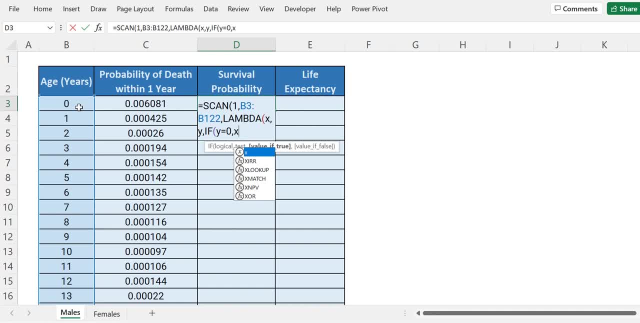 his age is zero. we want x back, that is one back, else we have to do x multiplied by now. this x is for the previous result that we arrived at right. so we are arriving at survival probabilities for age one. we are multiplying the previous result that we calculated with. 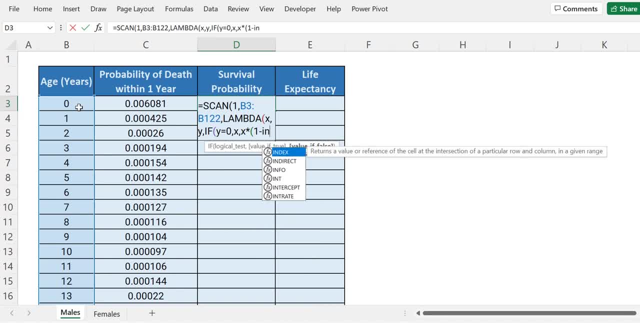 you the one minus. let's say we do index of this particular range, right, that is, probability of death within next one year and comma y. so we will take the current death of probability and we are subtracting that from one and we are multiplying it by the previous result, that is, the previous. 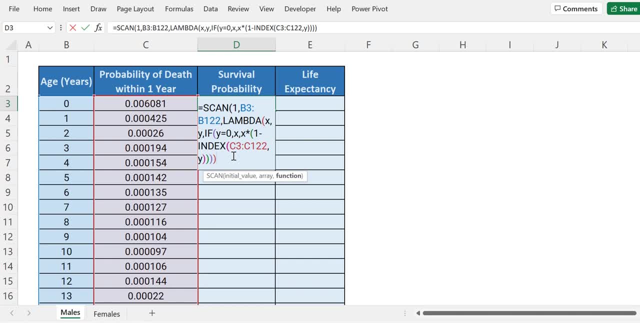 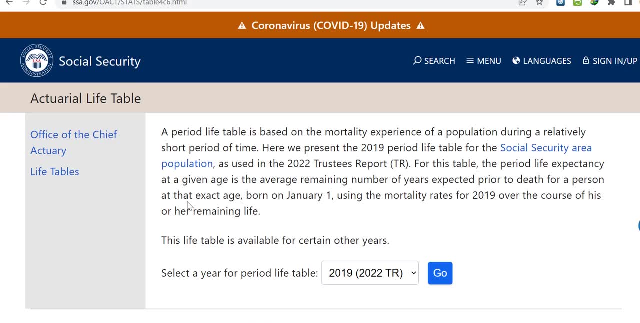 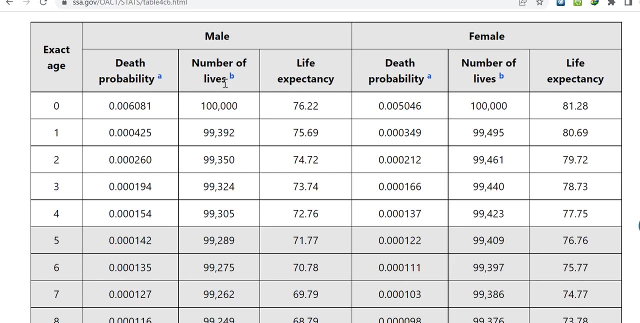 survival probability, and let's close the brackets and let's press enter so we have our results right and you can cross check these results from this website, from which i had taken this data. so this is the death of probability and this is the number of lives. so this is nothing but the survival probability, if you can arrive at survival. 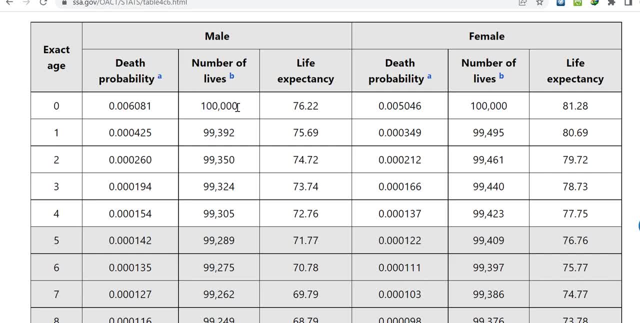 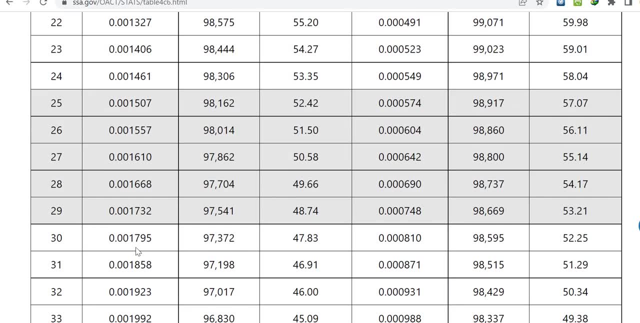 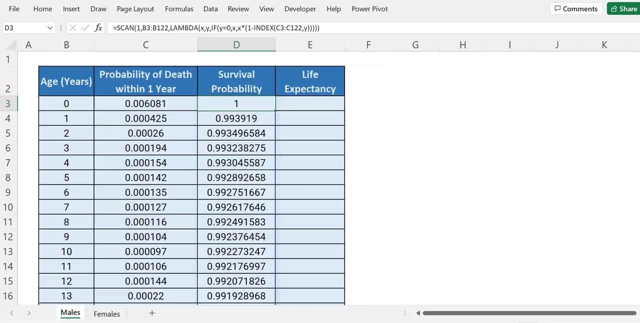 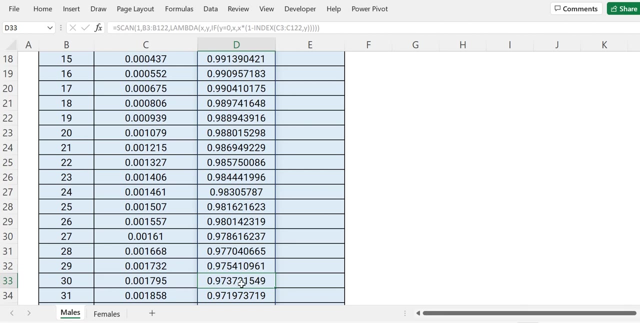 probability by dividing this number with one lakh, right, one lakh or a hundred thousand, correct? so let's say we check for, let's say, age 30, so for age 30 the survival probability will be 0.97372, correct? so let's check this. so let's come to age 30, and this is 0.97372, correct. so, as you can see, here we have 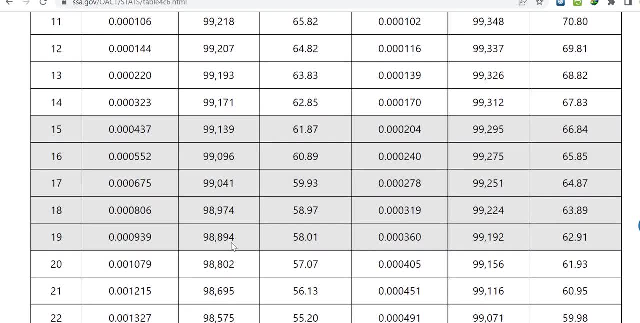 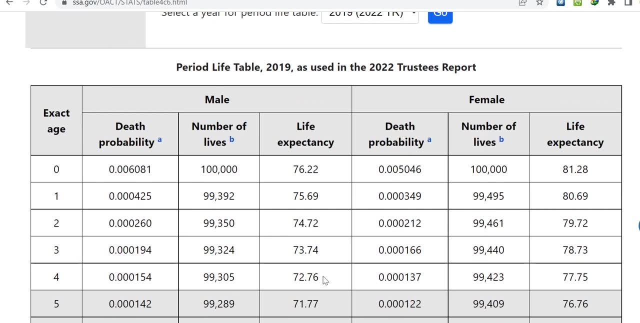 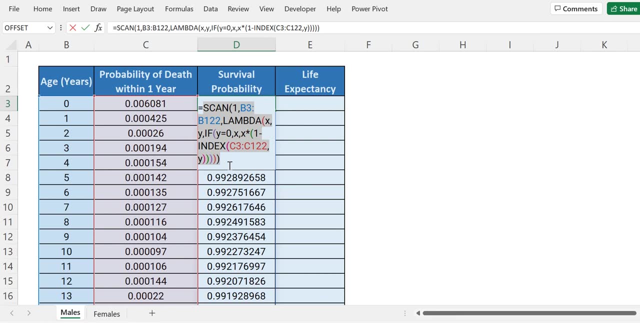 97372, right, so this one was for males and similarly, we have data for females as well, so this is for females. this is their death probability, and we have to calculate the survival probability in the same manner, so we will copy this formula. so let's copy this and, uh, let's. 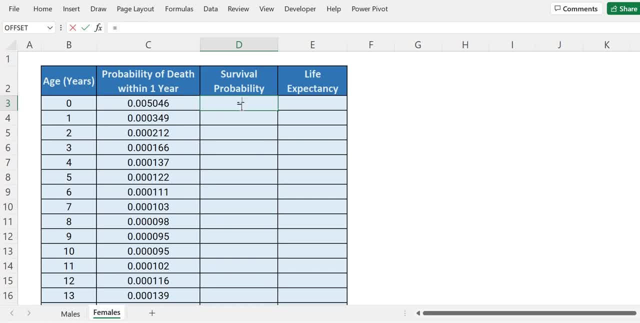 let's go to this sheet and let's paste it here. so equals to: and let's paste that formula, and as our structure is same, so the ranges selected are correct, and let's press enter, so we have the results for survival probability for females as well. right, and now we will have a look that how. 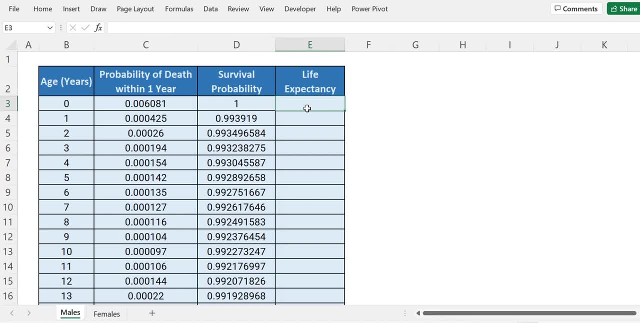 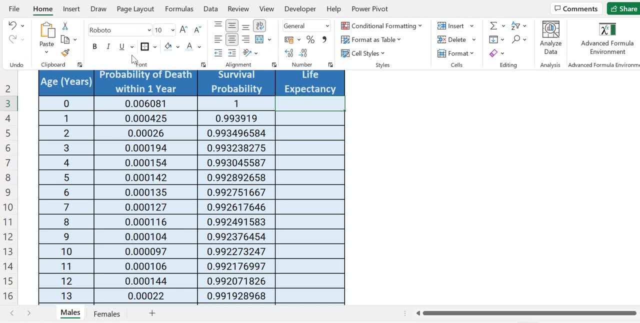 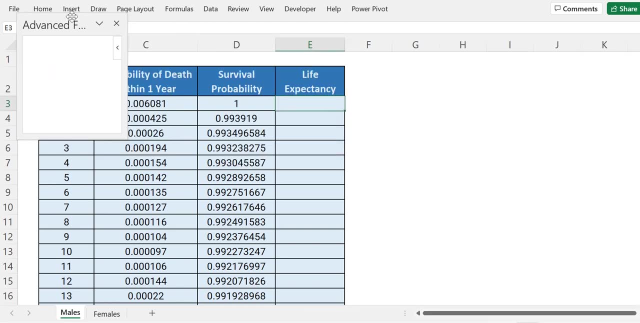 we can calculate life expectancy, so calculating life expectancy is a bit more complex. so i have already created a lambda for that and we can see that by going to home tab and going to advanced formula environment. right and now. this is the lambda, so i will attach the link of this, uh. 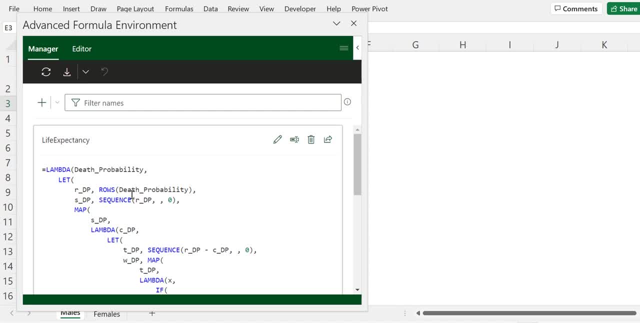 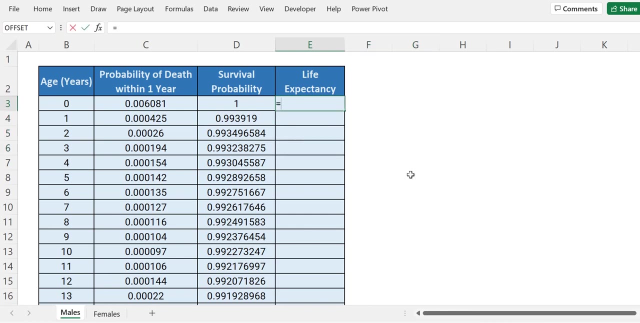 complete file in the description box. you can check out this life expectancy lambda and also implement this as well. so this is working fine. and now, now let's also test this. so let's close this and and here we will write. so here we will write: equals to life expectancy. so this is the 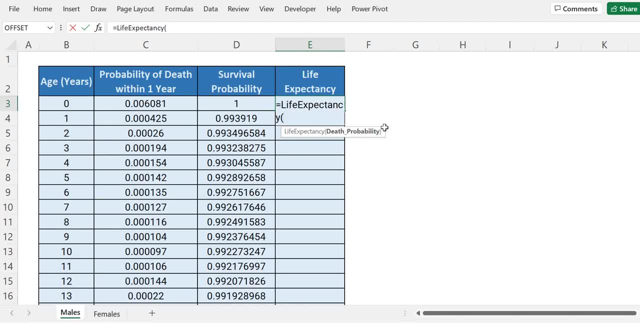 function life expectancy, and we have to just pass death of probability as our parameter. so we will select this complete range, that is, death of probability within uh, one year, and let's close the bracket, press enter and we have our results back right, so let's say we check. 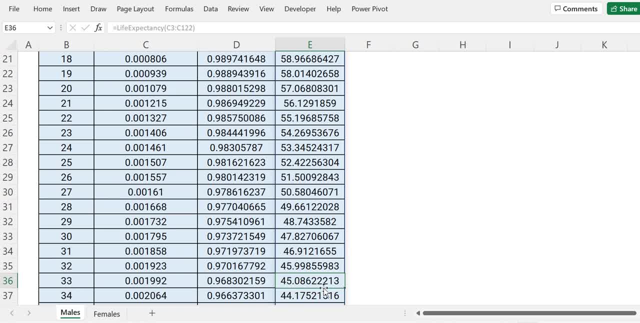 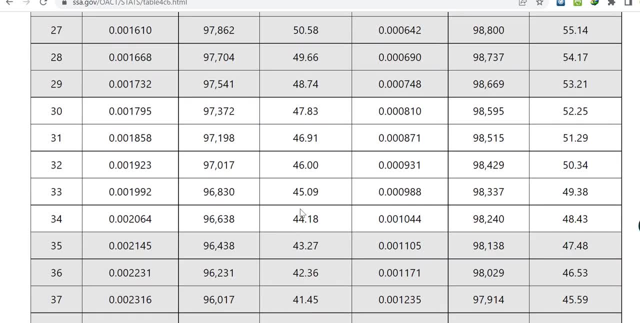 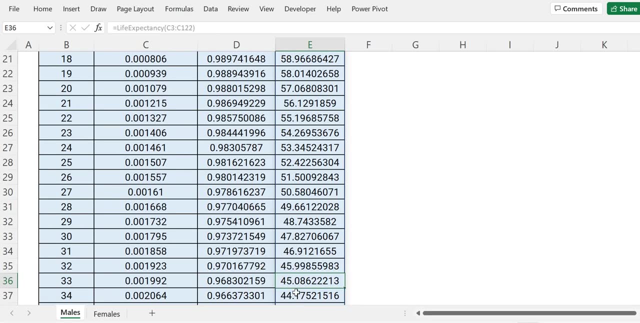 for- uh, let's say 33 this time, so this is 45.086, right? let's go to the website and we have to check for age 33, so this is 45.09. and let's check in our excel: so for age 33, it is 45.086. so if, if we round this to two decimal places, so this will become 45.09. 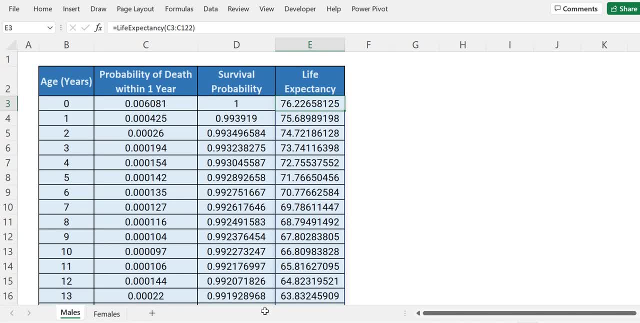 right. so this is absolutely correct, and let's also do this for females as well. so let's come here. and equals to life expectancy. so this is absolutely correct, and let's also do this for females as well. so let's come here. and equals to life expectancy, so 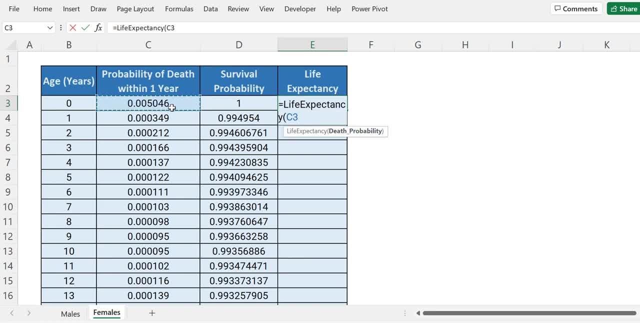 you can see that how easy it is to implement this is. there is no use of vba, just excel functions, right? so, uh, let's select this range and let's close bracket and press enter. we have life life expectancy for females as well, so these are the two functions that we can use to calculate. 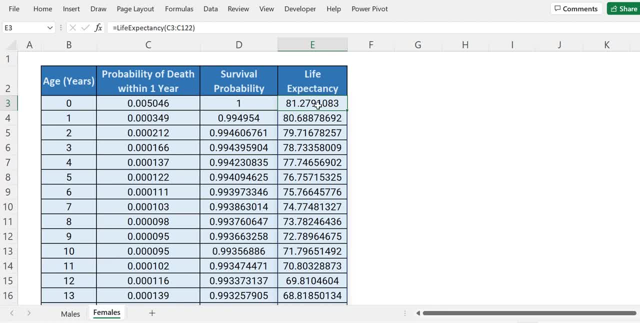 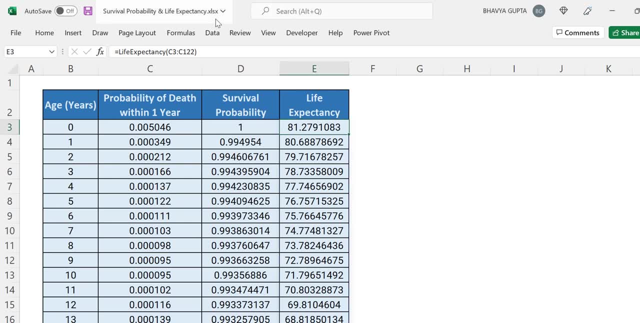 survival probability and life expectancy in excel and with no vba right. so as you can see that this is the uh, this is the extension of this file, that is xlsx, so no vba is involved. we have used only the functions that are there on the front end in excel. 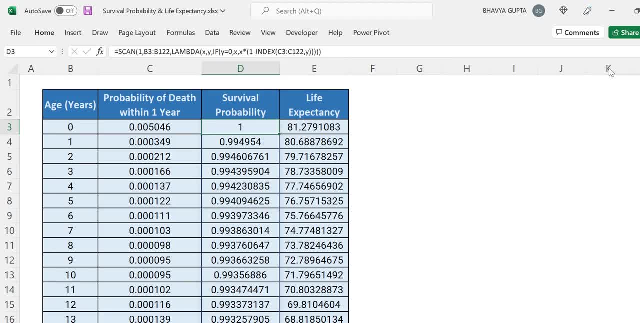 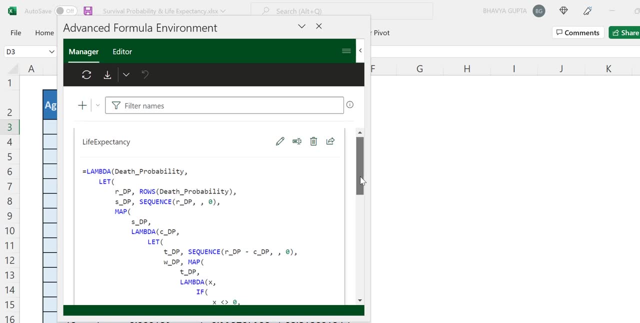 right, so you can check out this lambda as well. so, going to advanced formal editor, and you can check out this lambda for life expectancy as well, and similarly, you can create lambda for survival probability as well. and if you want me to explain that, how i created this life expectancy function, 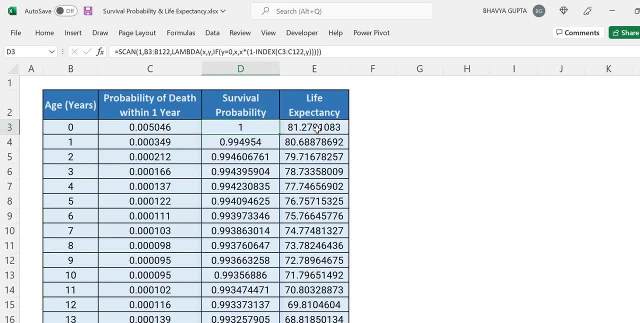 in excel so you can uh comment me and if i receive uh lots of requests for uh doing this, so i will definitely make a video right. so thanks a lot for tuning in, and that is it for this video. i hope you would like it and if you do so, please hit the like button and please. 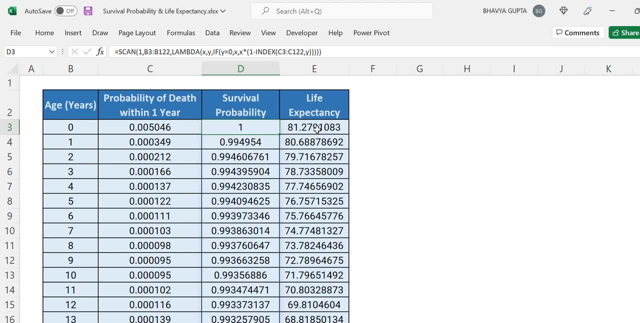 subscribe this channel for more such videos in future. so thank you. 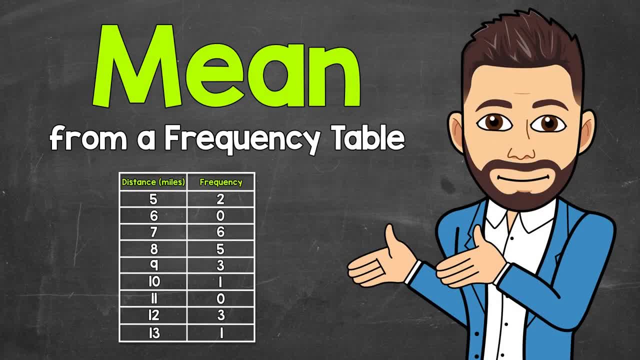 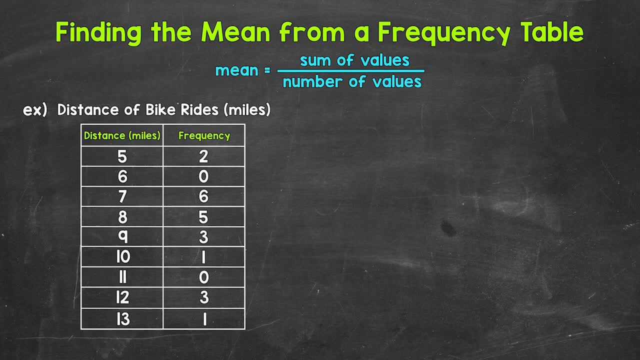 Welcome to Math with Mr J. In this video I'm going to cover how to find the mean from a frequency table. We find the mean by taking the sum of all of the values and then dividing that sum by the number of values we have. 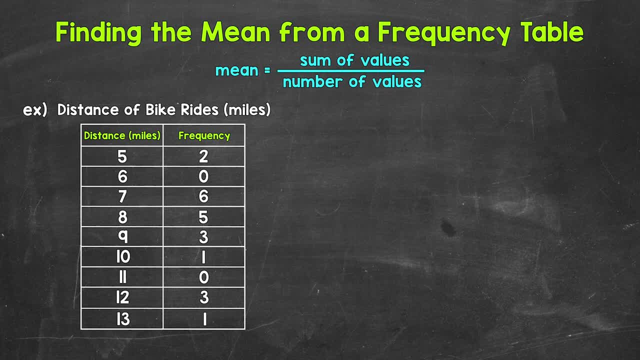 So add everything up and then divide by how many values there are. Let's jump into our example where we have a frequency table displaying data about bike ride distances. Let's say that a person tracked the distances of their bike rides for a month. These are the results In order to find